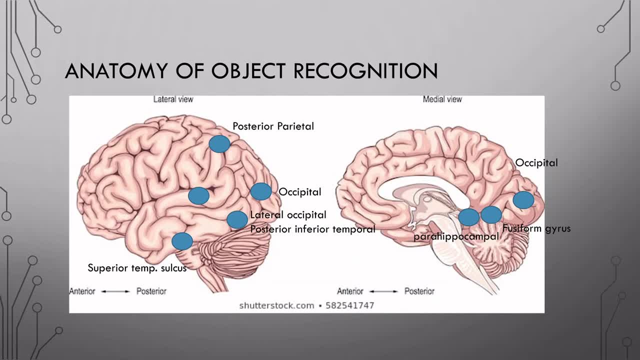 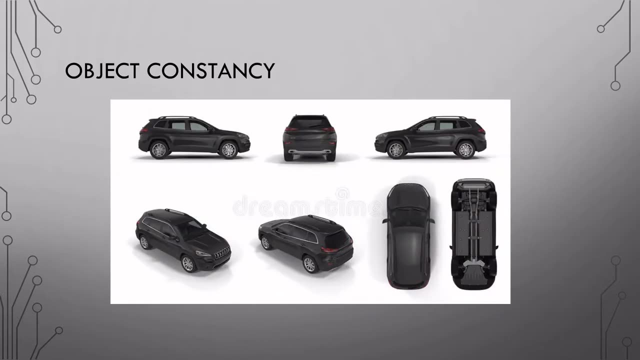 gyrus also help us to identify objects. So I know these are some pretty involved brain regions, but I just want you to be familiar with the names of these different regions in this object recognition network. These brain regions work together to identify objects, regardless of the situation. 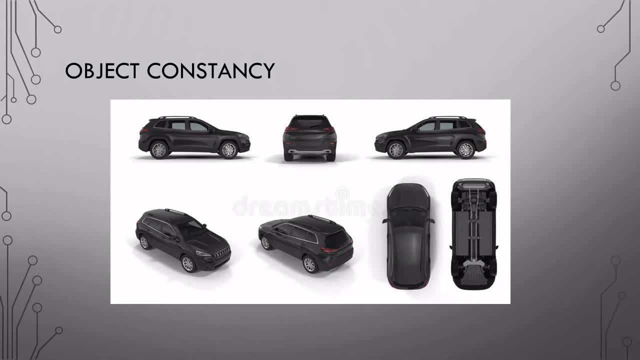 Object constancy is our amazing ability to recognize an object in countless situations. We can identify cars from different angles, or dogs, for instance, that are half in shade or behind a couch, partially hidden. Using this car example, our visual object recognition system still knows this is the same black car, whether we view it from the side or the top or the back. 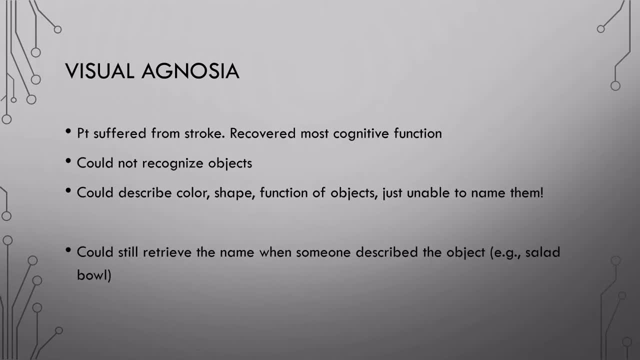 It's incredibly flexible in this way. However, I think one of the best ways to understand recognizing objects, or object recognition and its importance, is to look at cases where things go wrong. An example is a patient that suffers from a stroke. This patient mostly recovers all of his or her cognitive functions. language is normal, motor coordination is fine, visual acuity is intact. 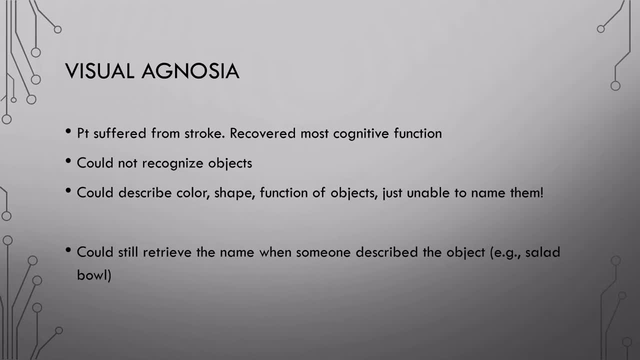 But they have a very specific deficit in that they couldn't recognize objects. He could describe the features of the object, like the color and the general shape of the object, but when shown actual household objects, this patient was unable to name them. He could describe the thing but not the name. and this case kind of gets stranger. 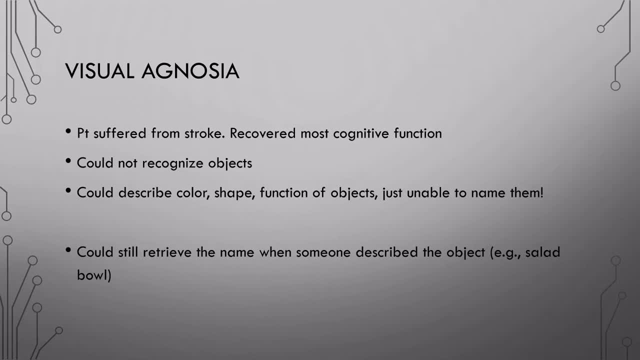 He could retrieve objects from memory just fine. so when asked to name a round wooden object in which lettuce, tomatoes and cucumbers are mixed, this patient said that's a salad bowl. But when shown a picture of a salad bowl, he was unable to name it or to identify it. 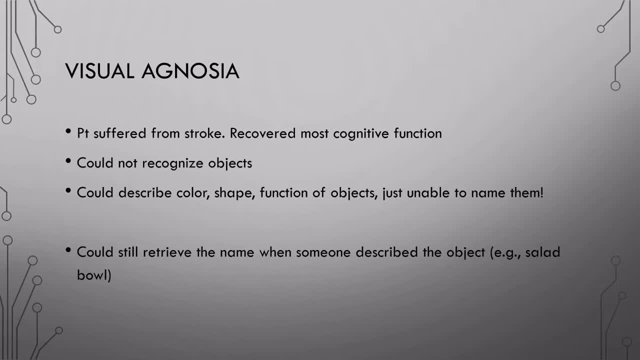 Failures of this kind are referred to as an agnosia. The A of this means kind of without, and the nosia means knowledge. So to be agnosic or agnosic- I think agnosic is the term to say it- means to experience a failure of knowledge. 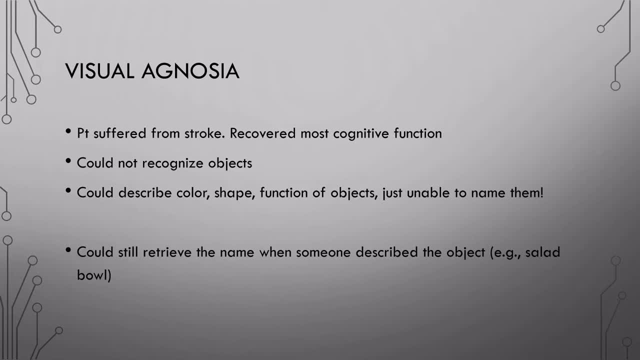 This patient in particular had vaginal agnosia, And this gives us a clue on some of the features that really underlie object recognition. So this patient could identify things by smell or touch through other sensory modalities, just not with visual cues. So we know that object recognition can come from different sensory modalities and that there can be specific damage to one or more of those. 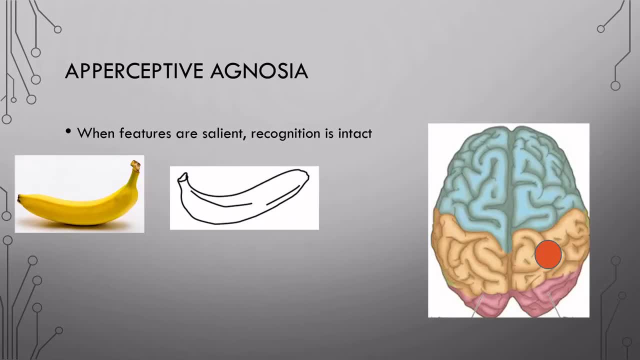 In this case it's visual agnosia. Let's move on to another type of agnosia. A perceptive agnosia occurs when a patient is still able to recognize an object, when the features are still really salient. So in the left picture of the banana the features are really realistic. 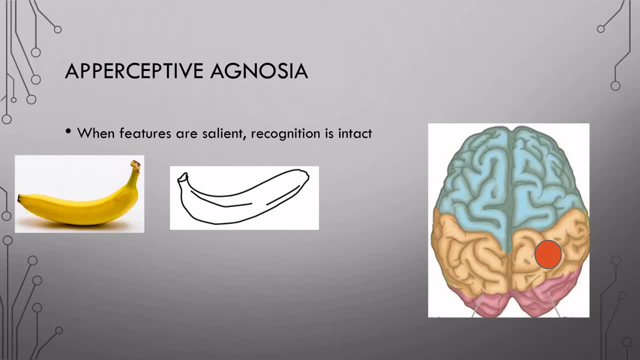 The color is bright and a patient could identify this banana. But the problem becomes evident when patients are asked to identify objects based on limited stimulus information, either because the object is shown as a line drawing or seen from a really weird angle. So this patient would not be able to identify the line drawing of the banana on the right. 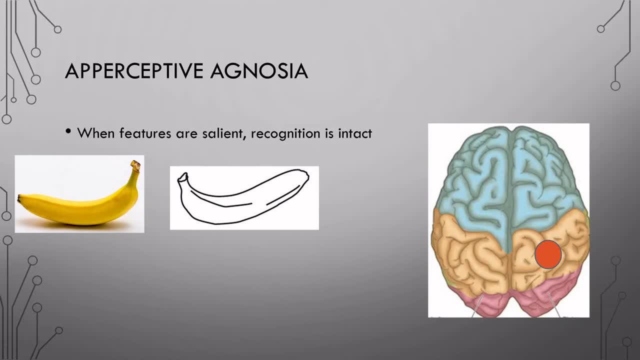 And this is a pretty specific deficit. This seems to be related to patients with damage to, specifically, their right parietal lobe, shown in the red dot here. Patients with right side damage have trouble identifying objects from unusual angles or perspectives, And a clue into this is because spatial information and integration is biased towards the right hemisphere in the parietal lobe. 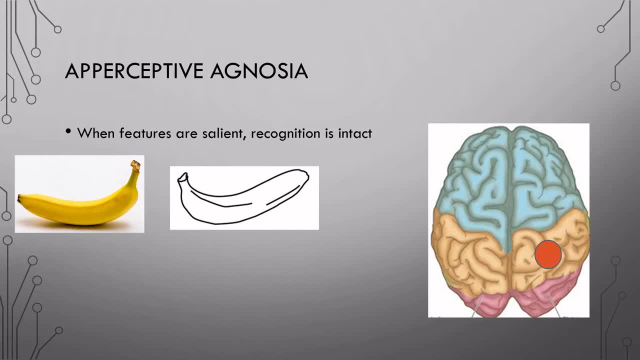 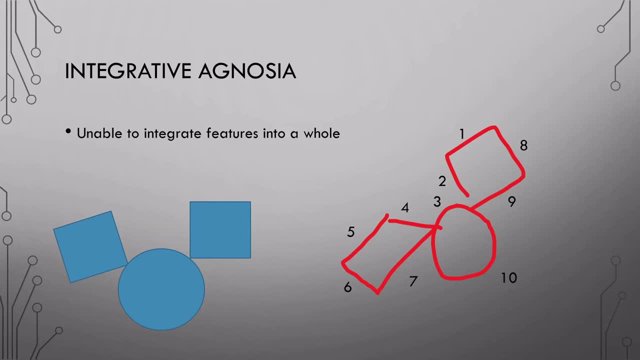 So this kind of becomes a problem of object constancy. Integrative agnosia is where a patient is unable to integrate features into parts or parts of an object into a coherent whole. For example, one patient with a head injury from an automobile accident was shown a picture of two squares and a circle in this particular arrangement on the left. 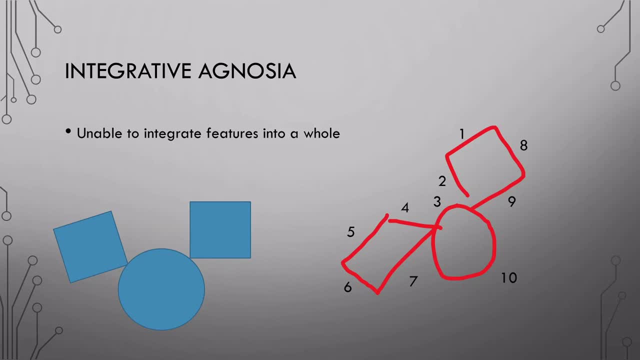 Researchers asked this patient to draw out the object. The picture on the right is an example of how the patient redrew this figure. But, interestingly, look at how this patient redrew it. The numbers on the right show the order in which they drew it. 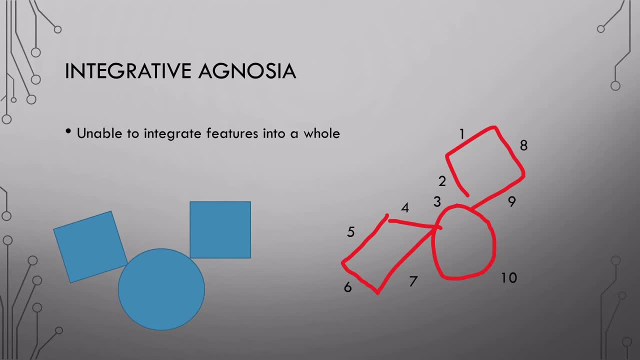 So he wasn't able to recognize that the figure contained two squares and a circle. Instead, he draws it as a whole, moving around the entire figure. This is an example of how patients with integrative agnosia are unable to identify or recognize parts or features within an object. 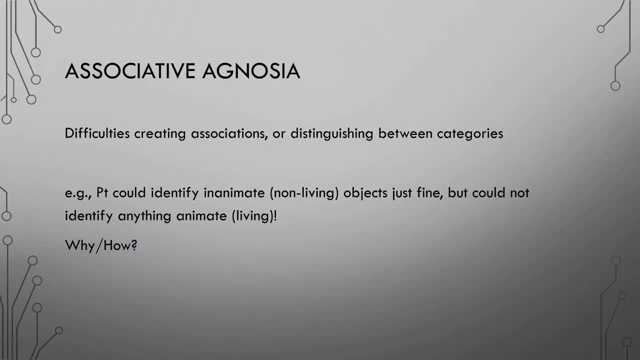 There are multiple types of associative agnosias, But it's mostly problems It can be caused with creating associations or distinguishing between categories. There is this bizarre case of associative agnosia where some patients cannot identify animate objects. So patients are just fine at identifying inanimate or non-living objects like chairs, tables. 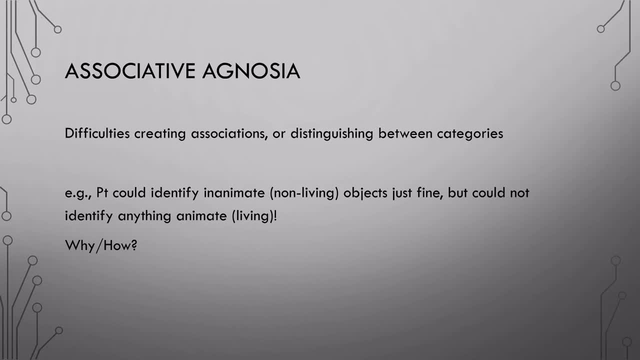 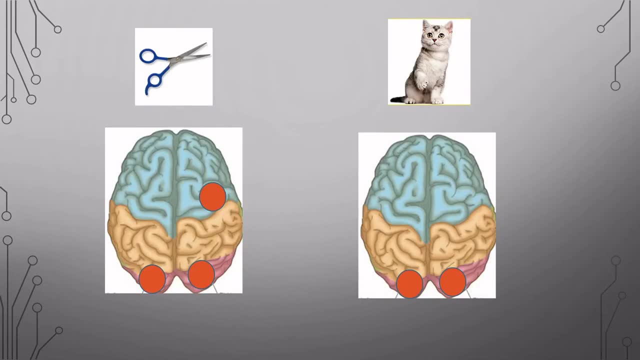 But when shown pictures of animate objects like a bird or a dog, the patient is just totally unable to recognize them. So how could this be the case? Here's some of the redundancy built into the brain while we think and process objects. Take a patient with damage in a part of the occipital lobe, thus giving him a type of associative agnosia. 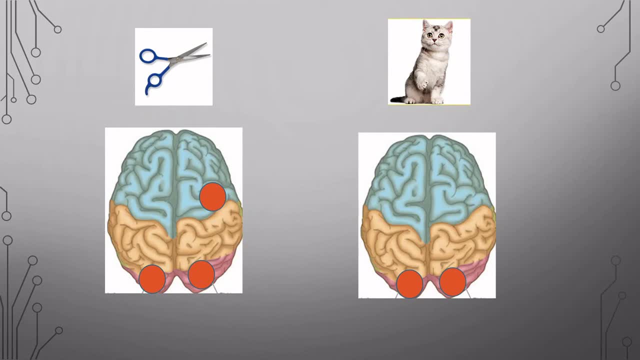 When shown a picture of a living cat, it is processed first in the visual stream or the visual system in the occipital lobe. Because of damage to that part of the brain, the patient is unable to identify the cat. But when shown a picture of scissors there could be additional processing. that's going on. 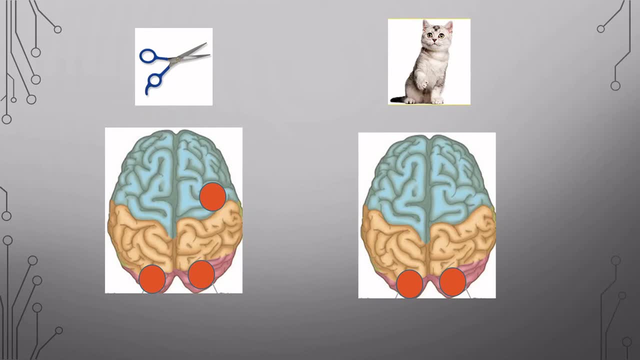 Initial processing in the occipital lobe would lead to a lack of recognition, like the case of the cat. But a patient might also imagine using this tool, So thinking about moving his or her fingers to use the scissors to cut. This would activate areas like the sensory motor areas in the brain as well. 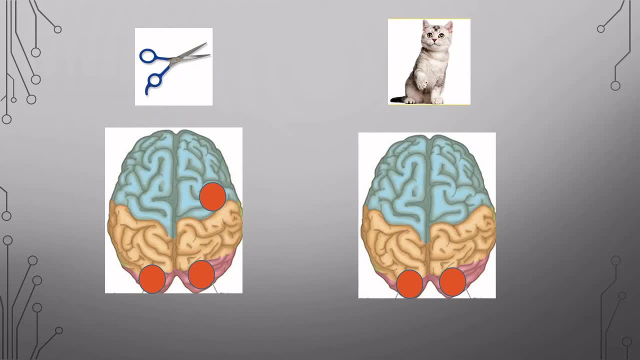 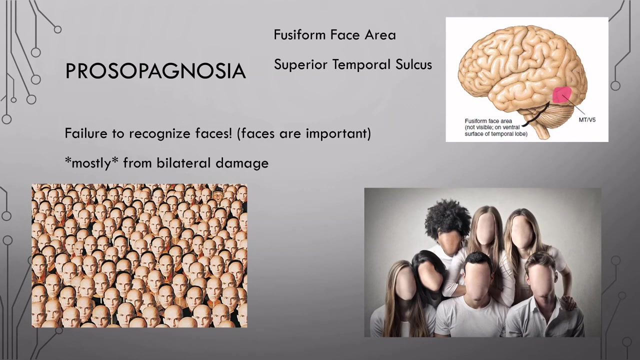 So this kind of additional processing would enable this patient to be able to recognize the object, even with an ability or even with an inability to identify animate objects. There's one last type of object recognition failure that I want to talk about, And that's prosopagnosia, or an inability to recognize faces. 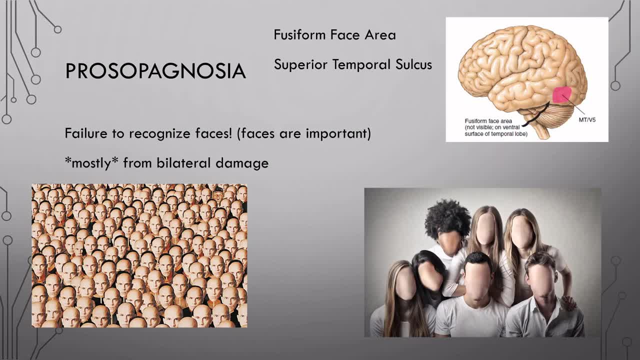 We take this for granted, but we rely on faces heavily to identify people. Faces are just incredibly important. When we meet someone or see a friend walking across the room, we don't look at their legs or the back of their hand to identify them. 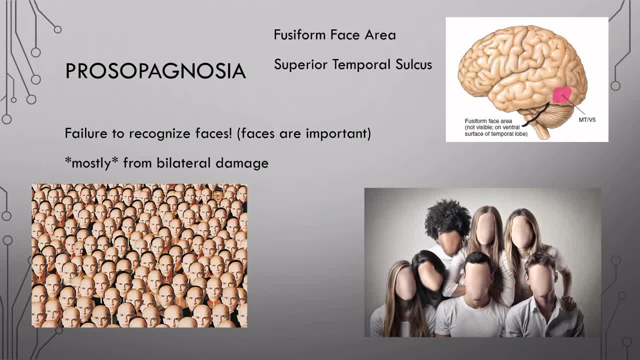 We look at their face as a cue to know. that's my friend, But there are cases in which people have lost this ability. Two areas are critical for face recognition, and that's the fusiform gyrus, or fusiform face area, and also parts of the superior temporal sulcus.